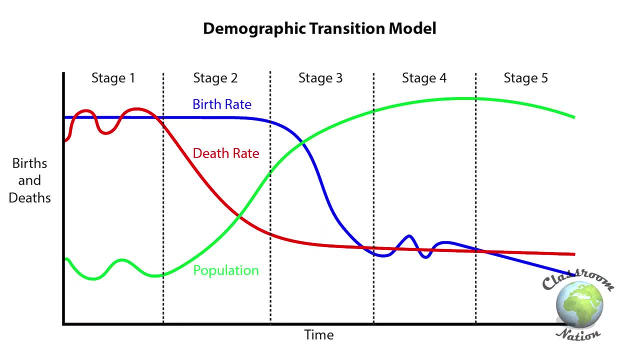 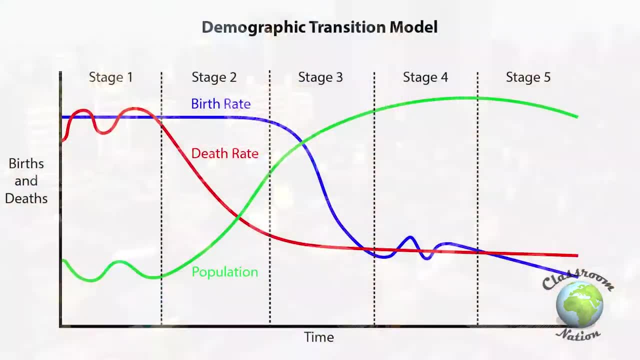 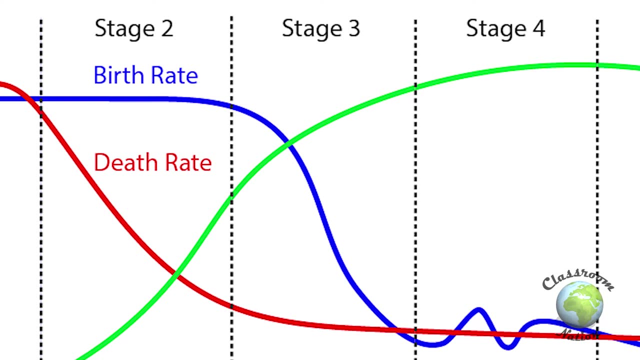 therefore, the population grows at an all-time high. people also start moving from rural areas to urban areas to achieve a better life. stage 3: late expanding stage: after a period of time, the social and cultural norms begin to adjust to a new, lower death rate. therefore, the birth rate begins to fall. 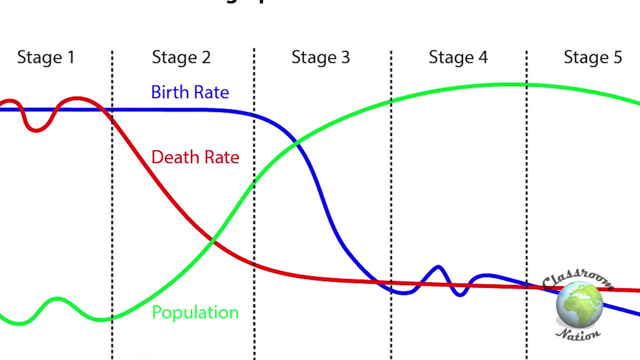 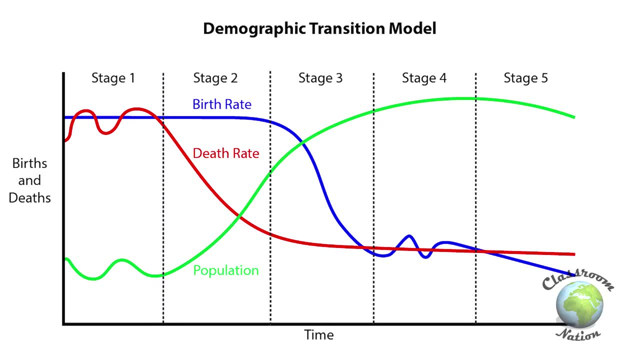 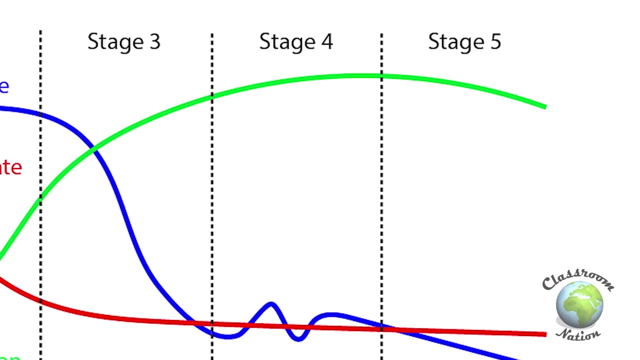 urbanization also begins to slow and the average life expectancy improves. infant mortality rate can be an important factor in the death rate growth and the overall quality of life continues to improve. stage four- lower stationary stage- both the birth rate and death rate are low. the population growth is very slow, if at all. the death rate may increase due to slightly aging population. 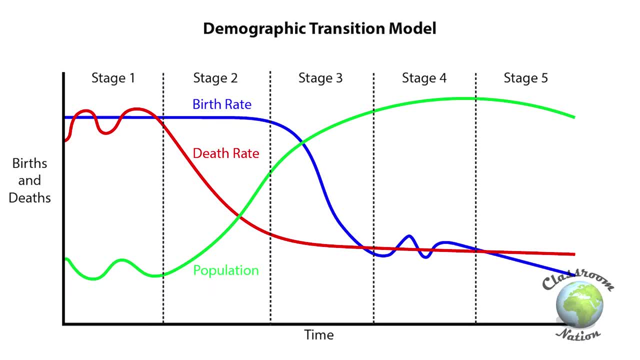 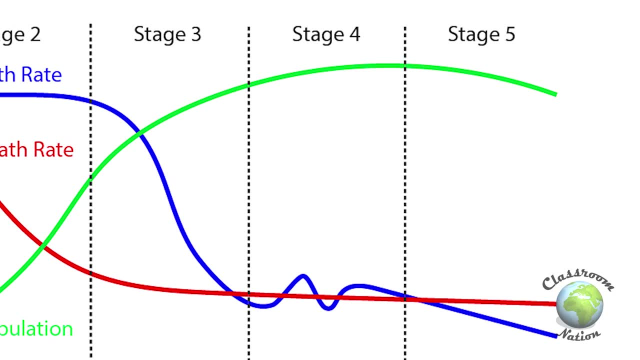 however, the overall life expectancy continues to increase. stage five: natural decrease stage. in the last stage, the birth rate falls below the normal death rate and this means the death rate is below the death rate for the first time. Therefore, the population begins to shrink. This can. 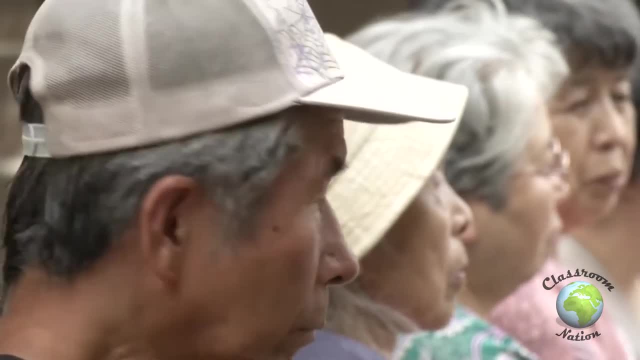 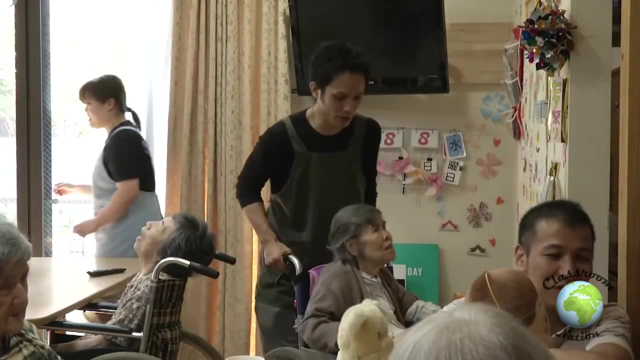 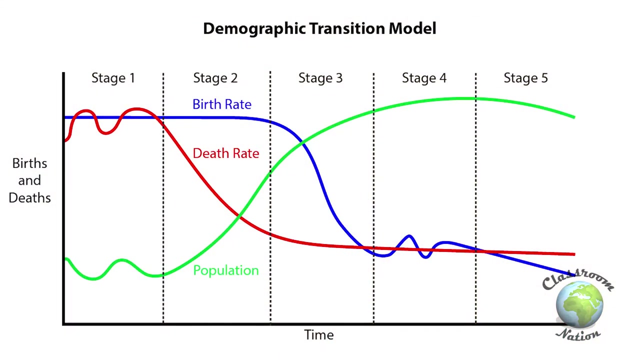 be seen in a few European populations and in Japan. In this stage, migration can become a very important tool for countries looking to balance their population demographics and introduce new, younger people into the society. One important thing to note with the demographic transition model is there is no prescribed 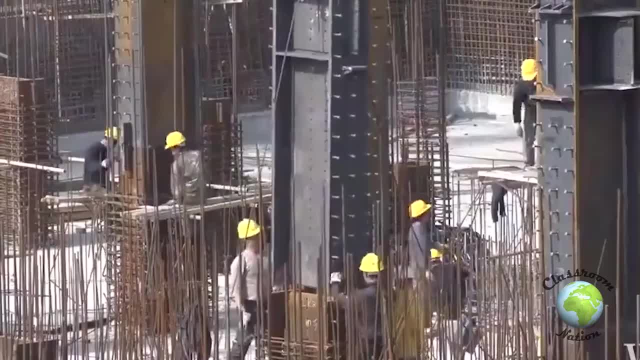 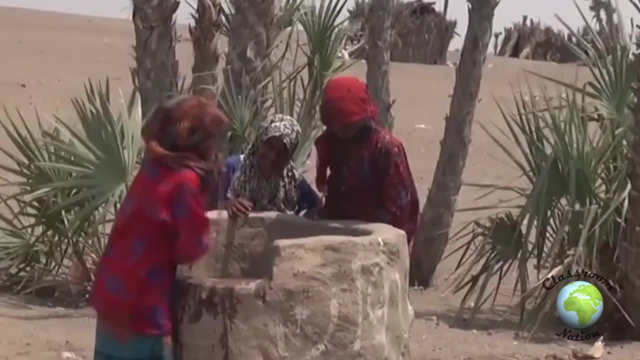 time frame. Some countries can move through this model very quickly, like China, for example, whilst other countries, particularly the sub-Saharan African countries, have struggled to break out of stage 1 and stage 2.. This is mainly due to disease outbreaks, political problems. 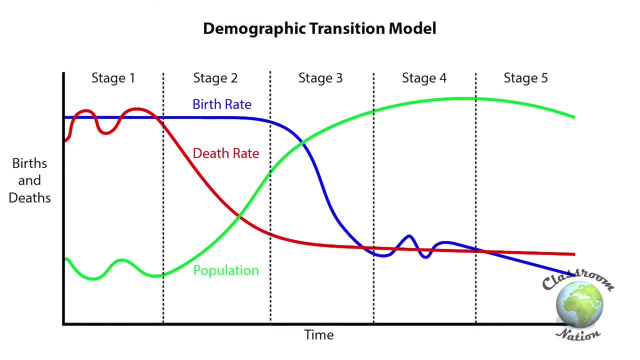 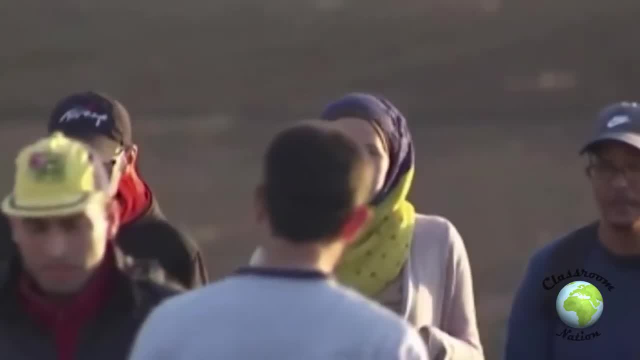 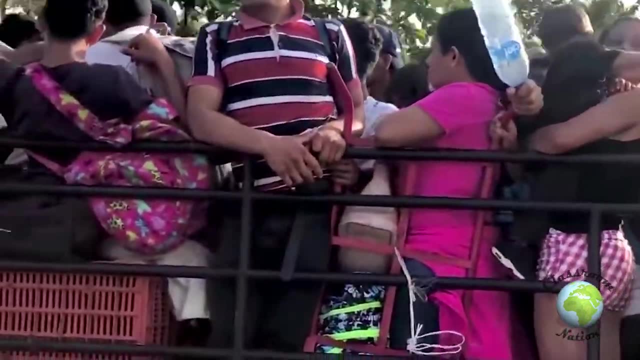 and instability due to war. Another important issue this model does not take into account is migration. Migration can affect populations in an enormous way. Outward or inward migration can change a population size and demographic. For example, many young adults migrate to other countries. 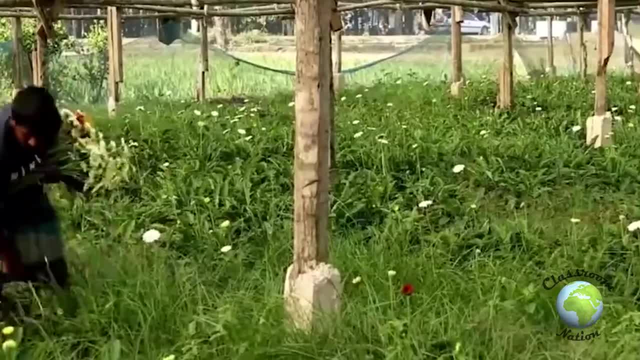 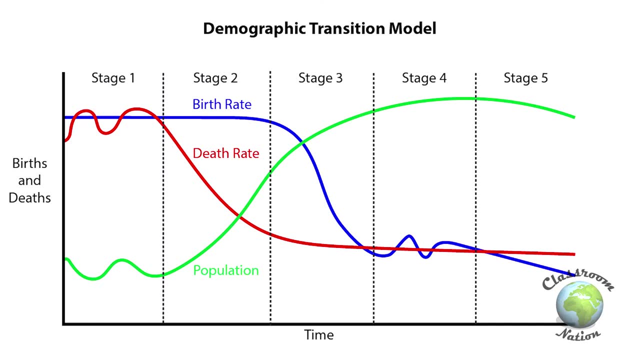 and therefore young adults, are more likely to increase the birth rate and maintain a population. In conclusion, the demographic transition model is a useful tool for looking at a country's development in a generalised, non-specific way, But there are some limitations. It is.